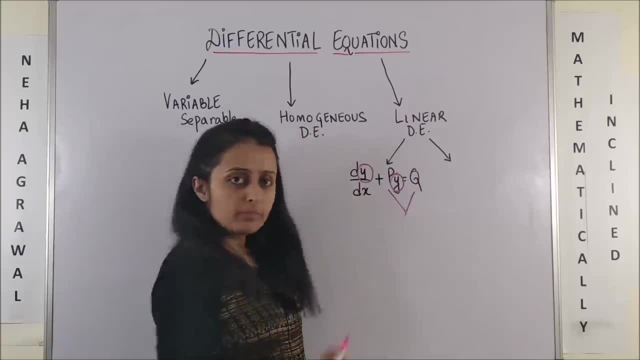 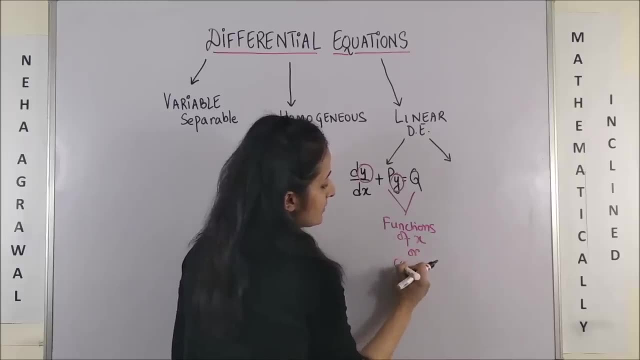 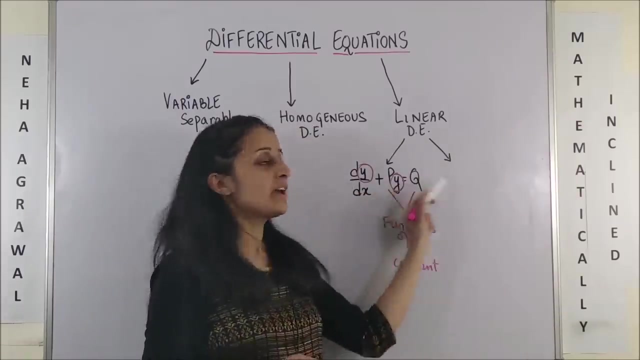 be y here, where p and q could be functions of x or constant Constant terms. Okay, Functions of x. Aisa zaruri nahi ki both p and q are functions of x, or both of them are constants. They could be one one each also, Okay. 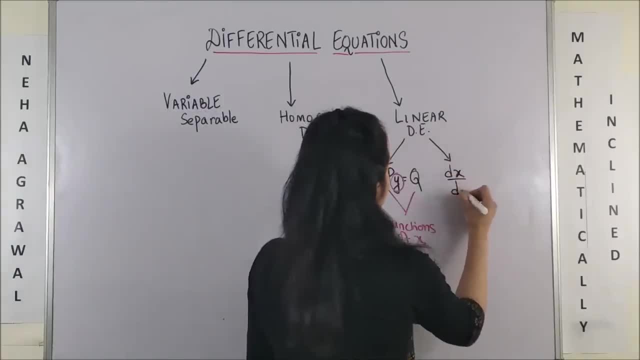 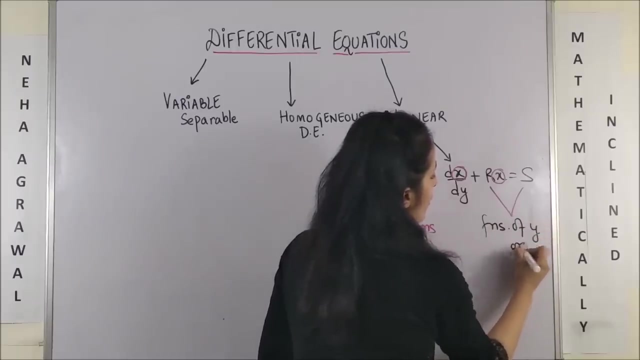 So, whatever, Agar ye nahi hai to. it is the second form, where Please see, Easy to remember If it's an x here, x here, And obviously where R and S, this time you would say, are functions of y or constant terms. Right, This is a background. Now the procedure. 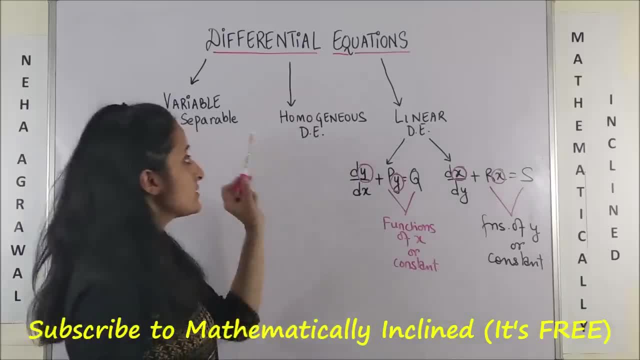 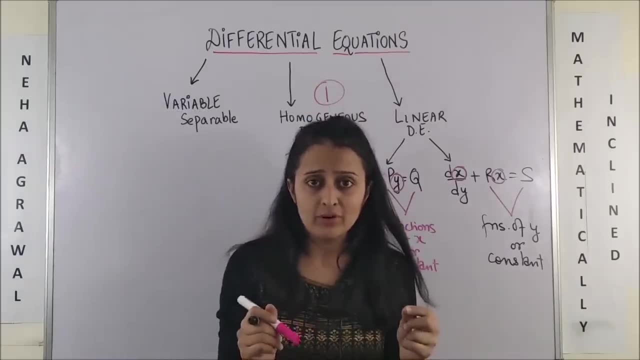 or the trick to identify the type of differential equation is always, always and always: First check whether it is homogeneous. Bohot simple hota hai, boss. I would share the examples. Basically, if each and every term is of uniform degree, woh? 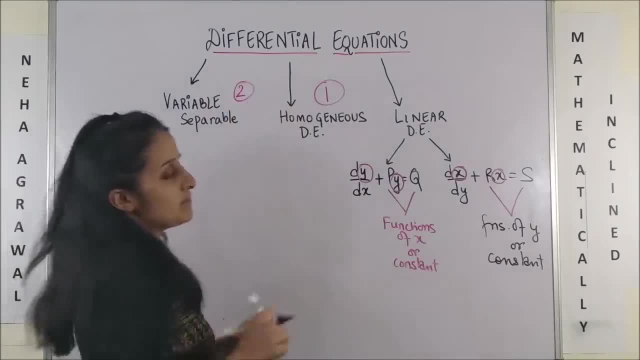 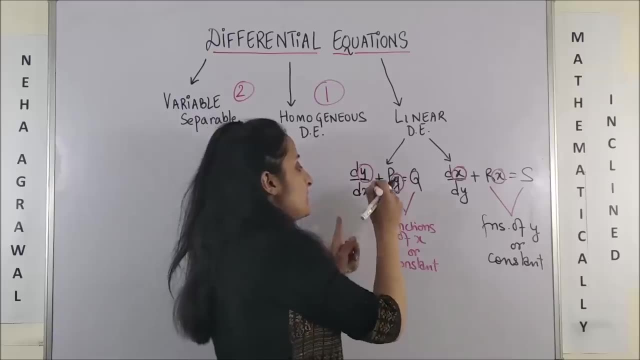 nahi hai, toh. secondly, move to variable separable. Can you separate them out? Yeh dono nahi toh. move to this form first, and yeh bhi nahi toh obviously it has to be the last one. 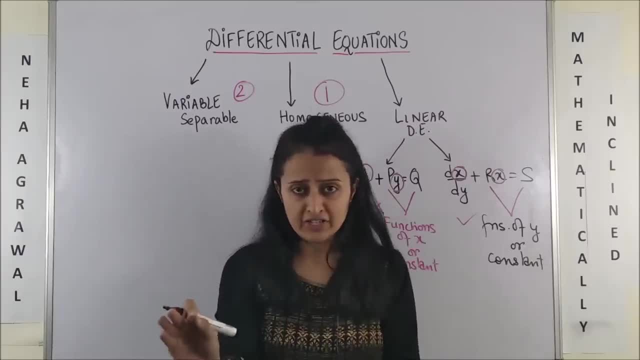 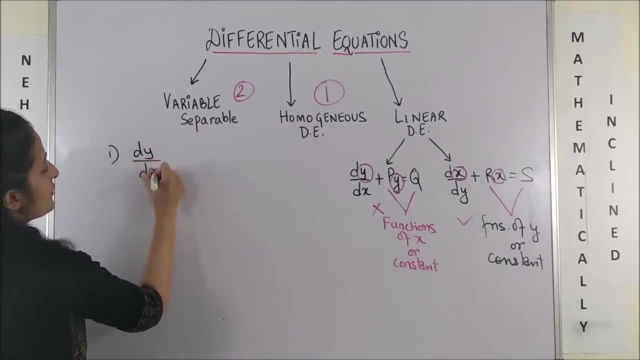 Please remember, before you begin with any differential equation question, where you have to solve it. first and foremost step is write everything in terms of dy by dx is equal to the function. Jitna marzi complicated ho. write it this way. Second step: 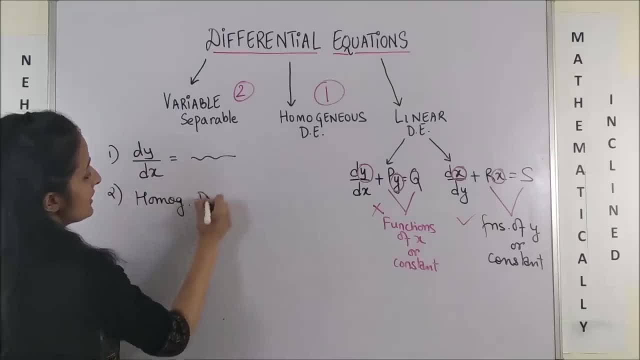 check for homogeneous differential equations. Agar yaha se mila no, then you go for variable separable. In case this is also a no, then move to linear differential equation type 1, which is this: Nahi, toh, just flip this reverse. 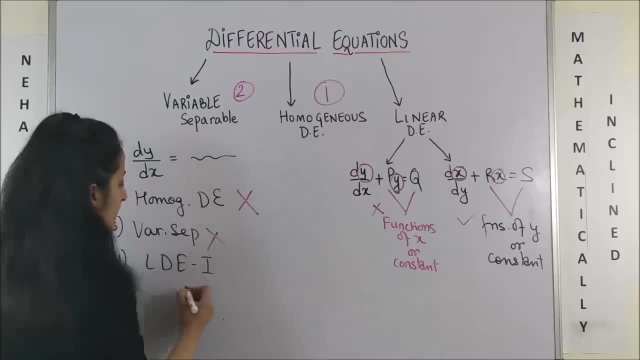 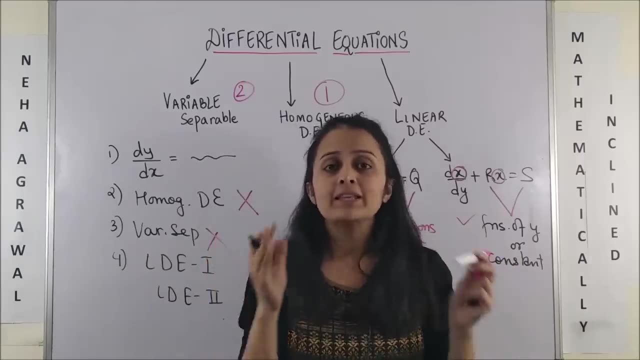 both the sides. Okay, so just flip both the sides and write: linear differential equation 2 form: Kuch na kuch toh hoga, hi boss, Make a note. and then let me take some examples. Chaliye ji lagate hain. 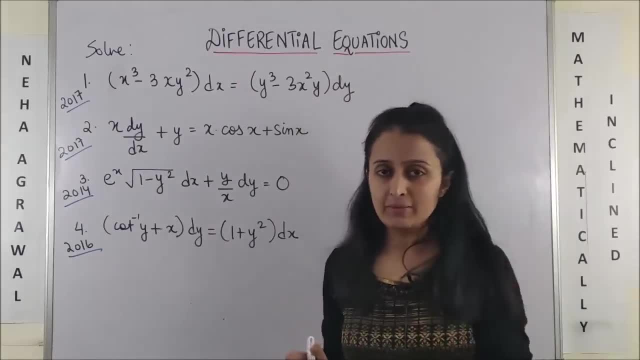 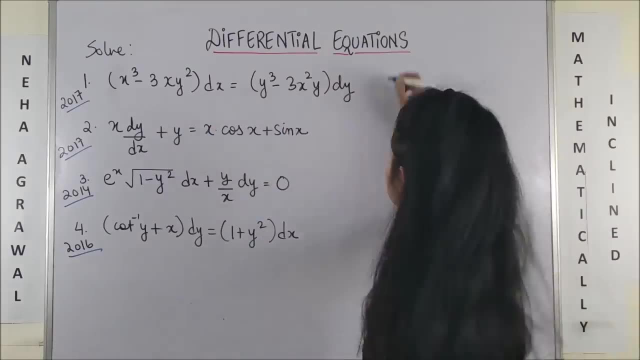 apna ramban ilaj. Looking at the first question, came in Delhi 2017.. This is the equation. Step 1, write everything in terms of dy by dx, So this will become: dy by dx is equal to x cube. 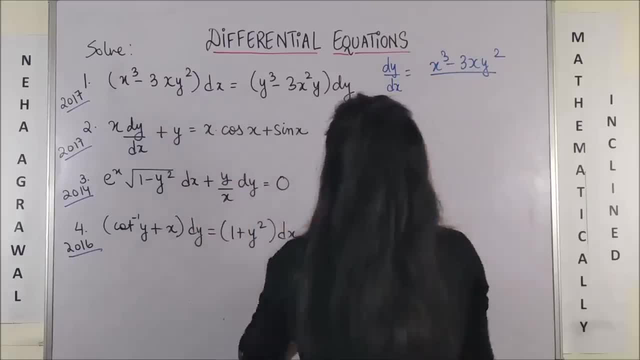 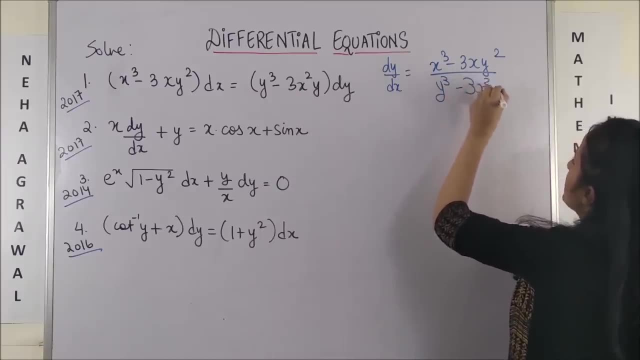 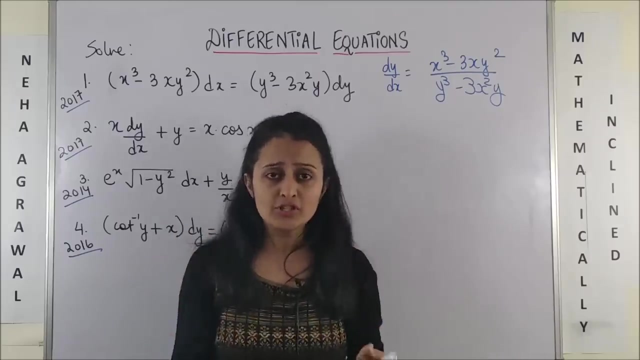 minus 3xy square upon, I have y cube minus 3x square, y Chike ji. This is the equation. Now, as I told you, first check is it a homogeneous? So this means: look at this term: x, cube, matlab, degree 3.. 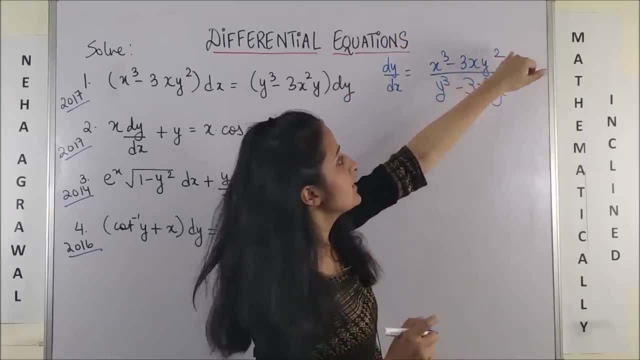 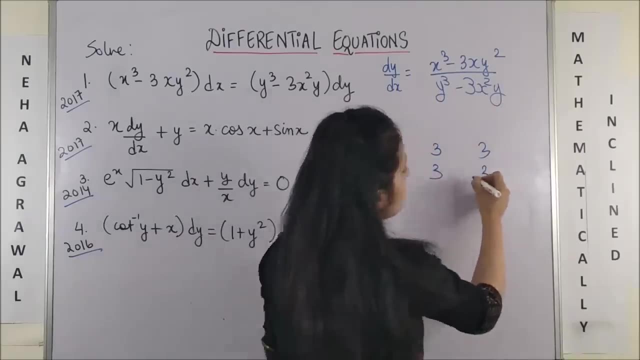 Look at this term: x has degree 1, y has degree 2.. Add it together: degree 3.. y cube degree 3, 3x square y: degree 3.. Toh bingo Hai na sab, degree 3.. That means: 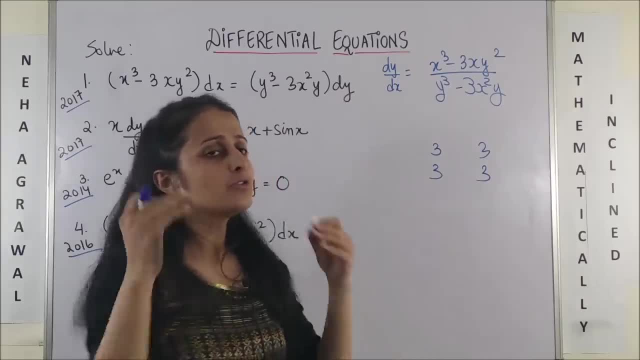 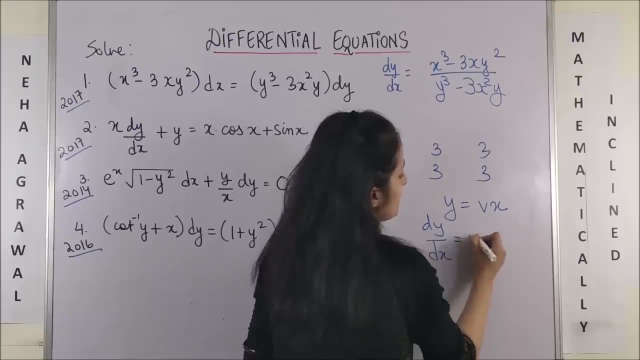 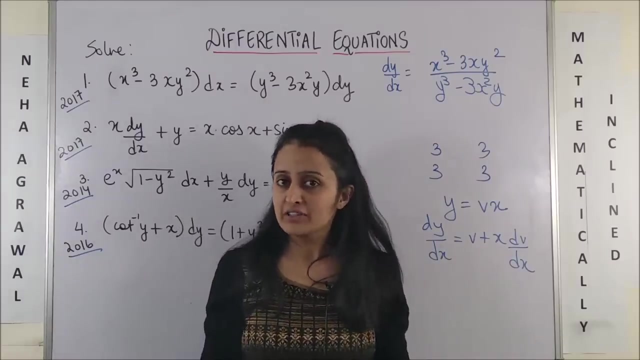 this is a homogeneous differential equation. Now you are free to write this: as y is equal to vx, Then this means dy by dx is equal to v plus x into dv by dx. Boss, solution mein nahi jaari, If you really want to learn how to solve a differential. 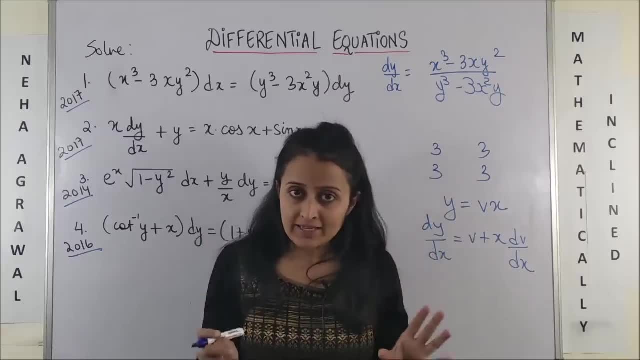 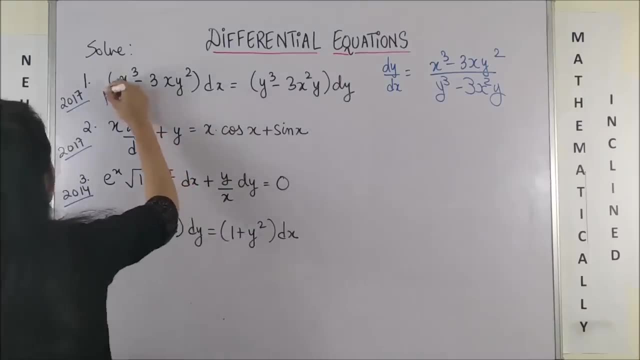 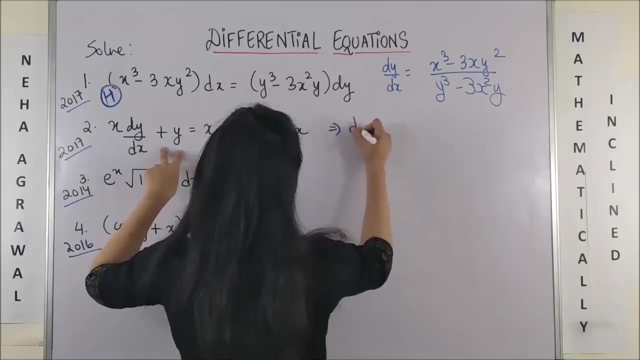 equation. click on the i button. You can check the playlist. differential equations. jisme hai video solving homogeneous differential equations. So the first one was homogeneous, Next one: now again we have to write our dy by dx. So to simplify, this will be dy by dx is: 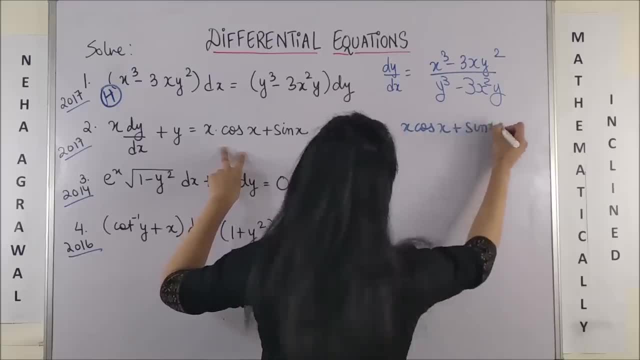 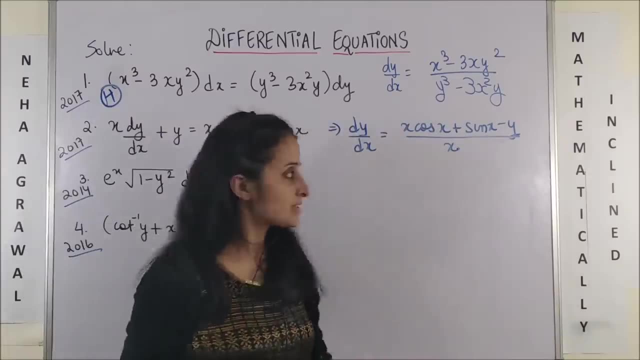 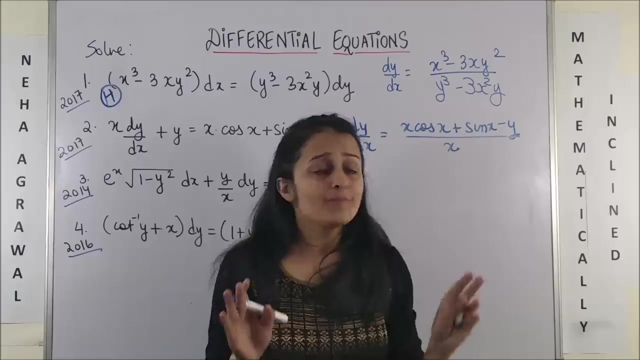 x cos x plus sin x minus y, and this is upon x, so upon x. Now, this is how my dy by dx looks. Now, this is x cos x. this is sin x, y, x. all of them are varied degrees, right? So basically, 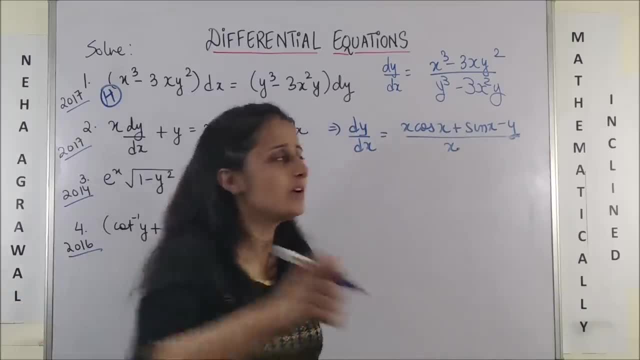 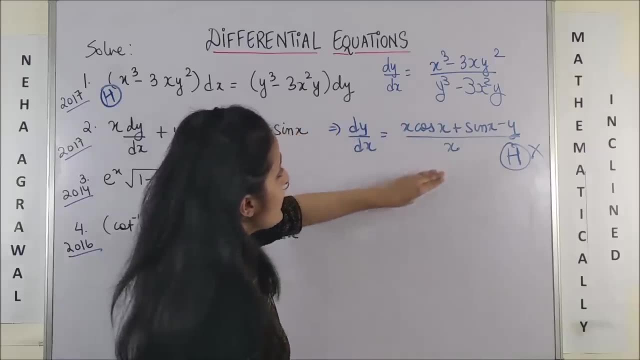 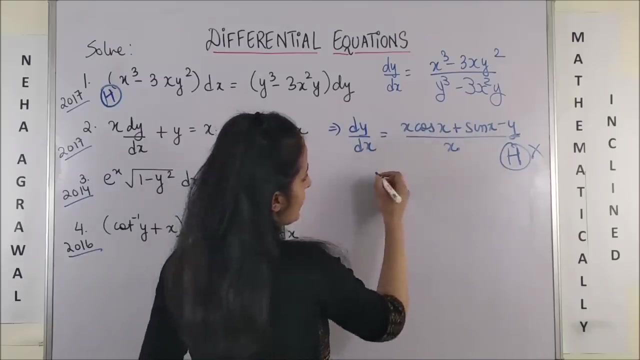 in sab ki degrees hai different. it cannot be homogeneous. So homogeneous differential equation is out of question. Moving next, let's see if I can separate these out. Separate means if I combine all the terms containing x on one side. If I take my dx on this side, this 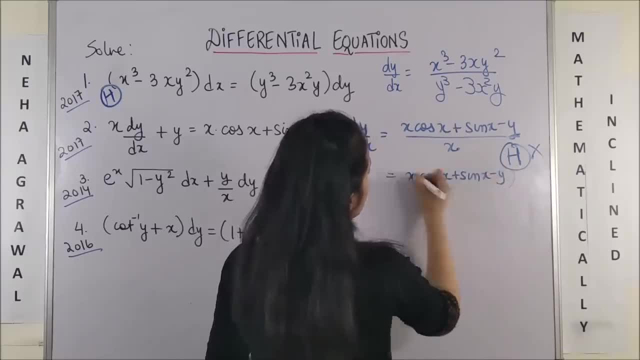 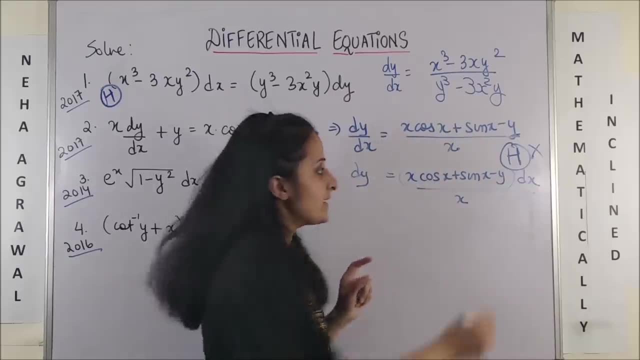 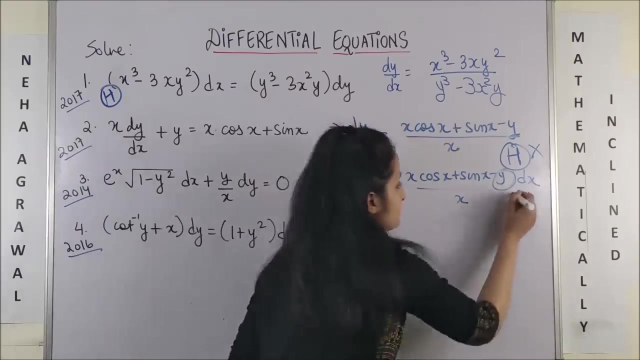 is x, cos, x plus sin, x minus y, whole dx upon x, and this is dy. Now, although all other terms are in x, but is y ka? kya kare? I cannot bring it down without getting dx To matlab. ye separate bhi nahi hora. 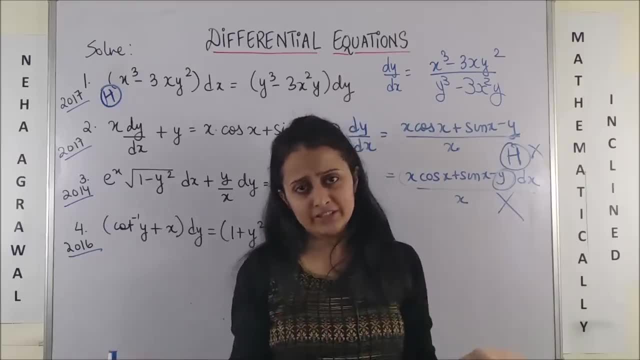 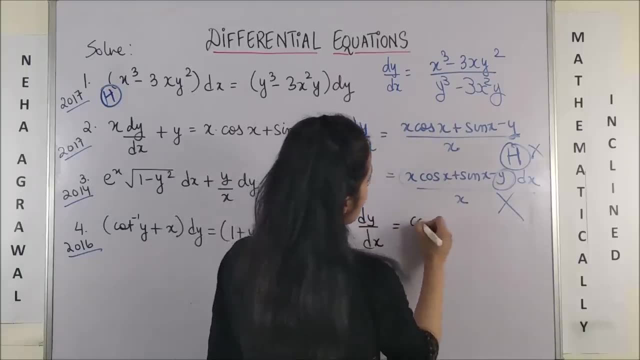 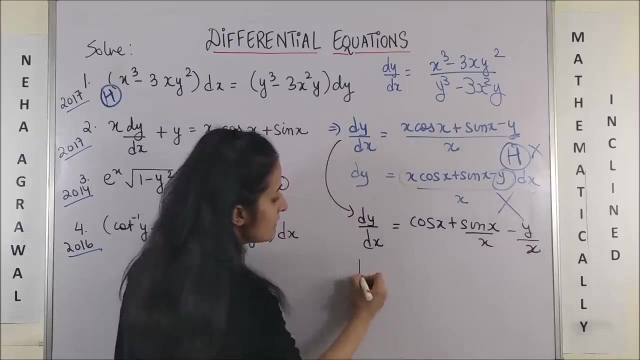 That means I am left with the options of linear differential equations Coming to the first one. so from here, if I say dy by dx is equal to cos x plus sin, x by x minus y by x. Isko thoda sa, we will try to. 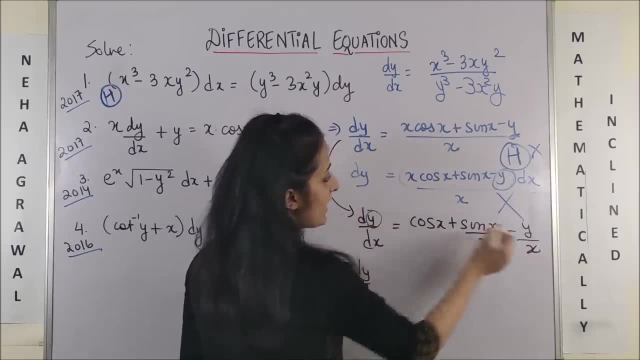 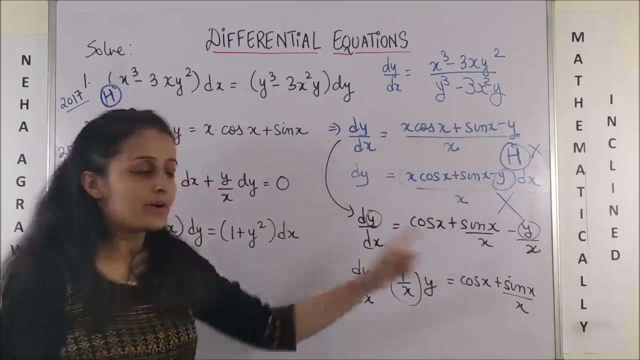 bring it to the format So dy by dx. You remember we had y and y connection, plus 1 by x into y, because it should resemble: py equal to q is equal to cos x plus sin x by x. Thike ji Ab ho gaya apka. 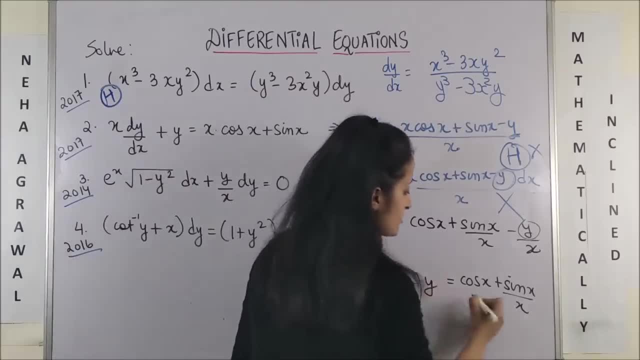 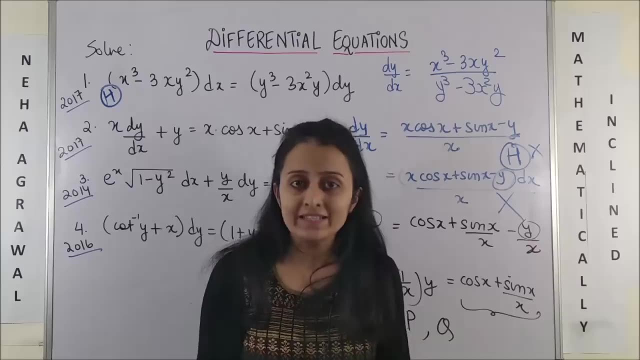 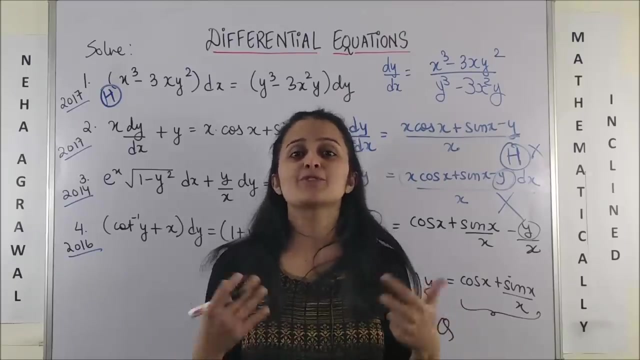 linear differential equation, where this is p, a function of x, this is q, again a function of x. So, in these cases, what do we do? We find the integrating factor. Ok, so we will do that and proceed. I am planning to upload a video on solving. 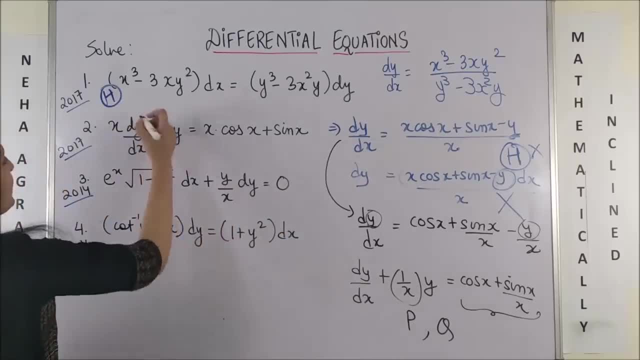 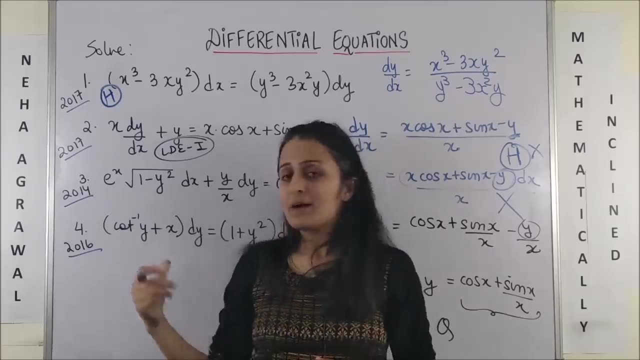 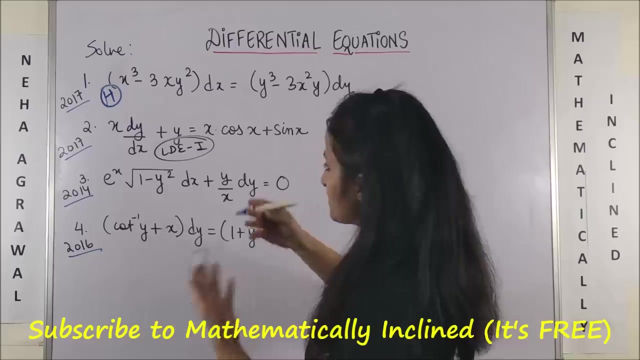 linear differential equations soon. Alright, so we have identified. this is linear differential equation type 1.. Make a note and then we will discuss what happens with third and fourth. Ok, now let's look at the third question. Same logic. let's express dy by dx. So this will be e raised to: 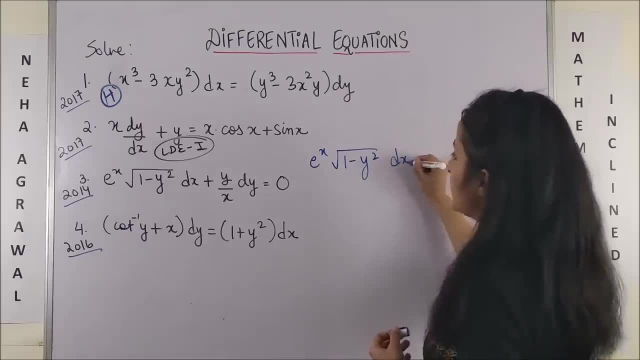 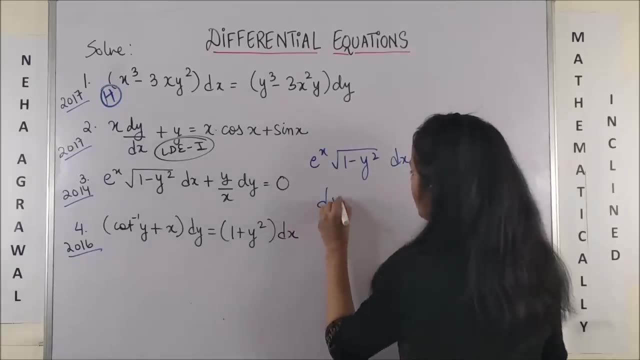 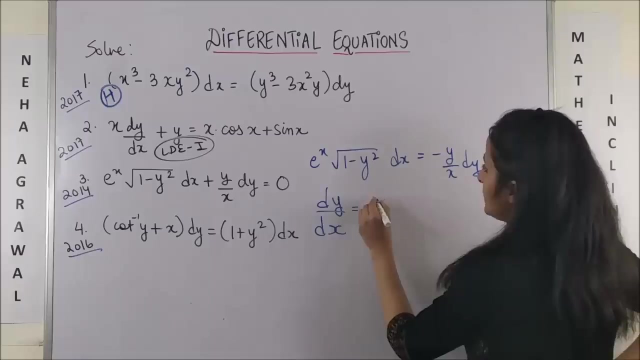 power x into root of 1 minus y square. dx is equal to minus y by x dy. Ok, so this means dy by dx is equal to with dx. I have this, So I will get e raised to power x into square root of 1 minus y square. 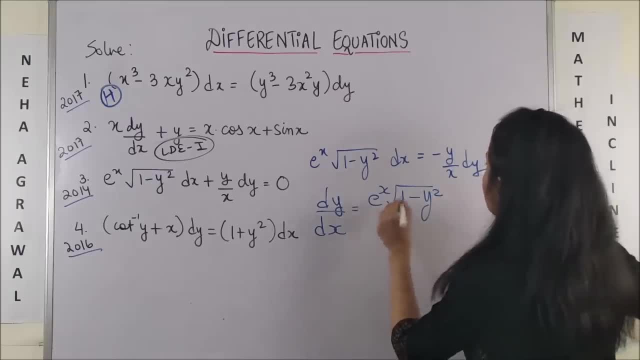 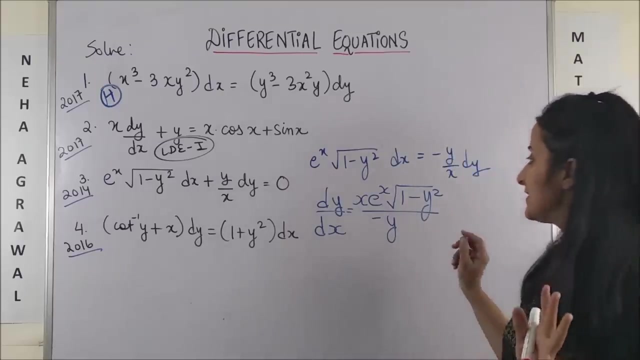 Alright, and here I will have into x upon. I have this minus y. Ok, now, this is what I have. Now. please look at each and every term, Boss. I don't see this homogeneous anywhere. You see x, e to the power x, then suddenly 1 y square. 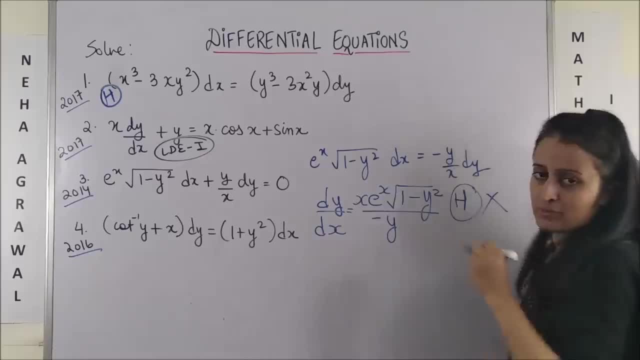 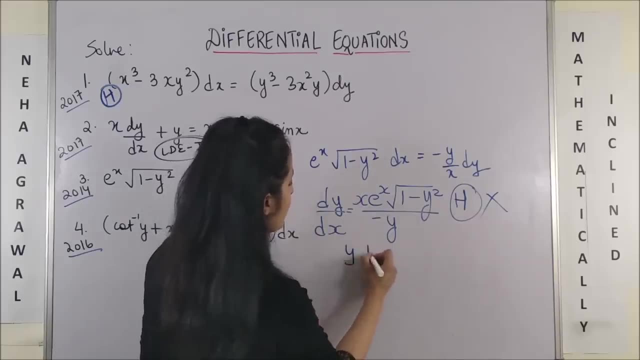 y. So not homogeneous, boss. Then let's try. if it is variable, separable, That means, if I can get my dy here. so y into dy is equal to e to the power x, and this also can be moved here, and this is e to the. 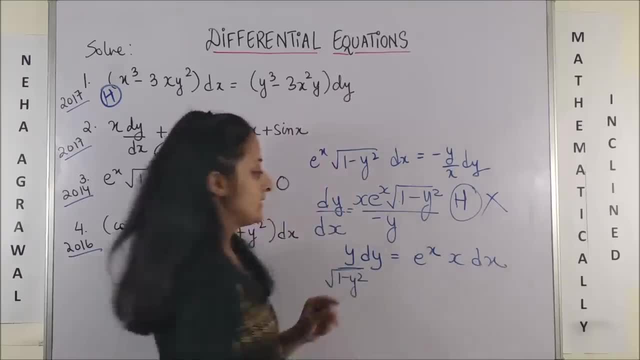 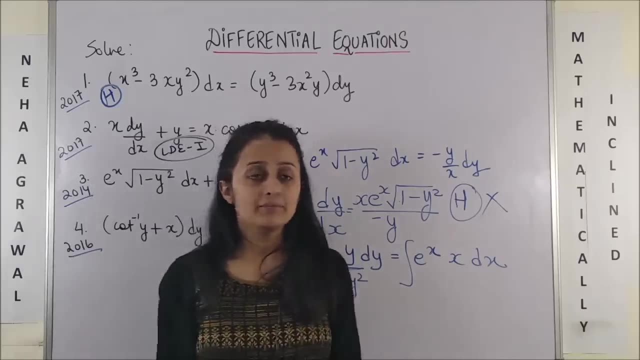 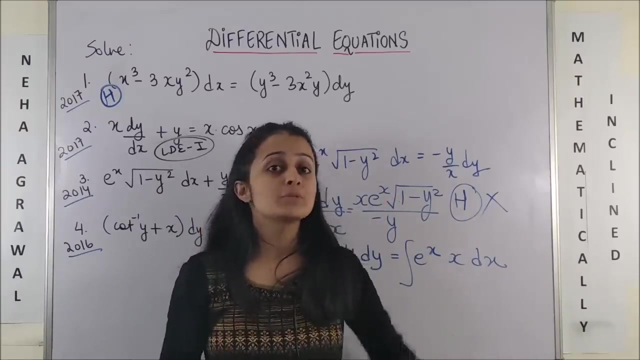 power x into x, dx, Right, Yes, I could separate them out. Now, if I want, I can integrate them. This is everything in y. This is everything in x. If you want to know how to solve variable separable forms, again go to differential equations. 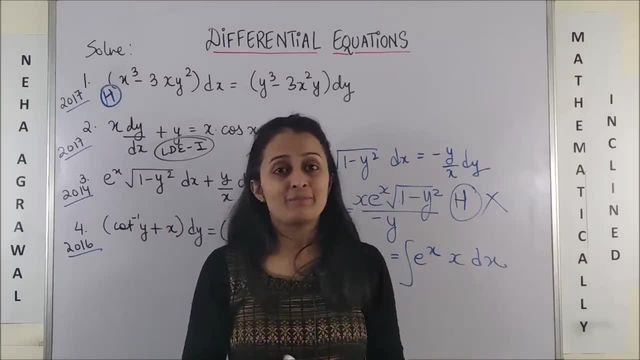 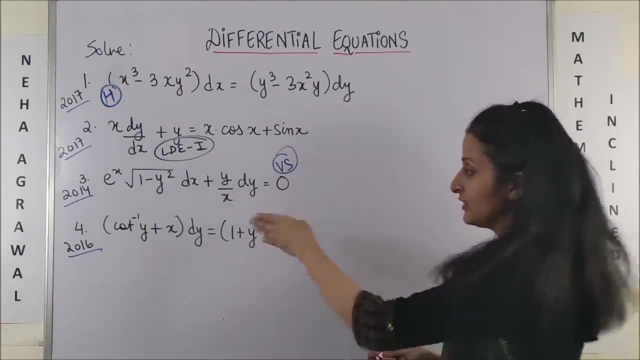 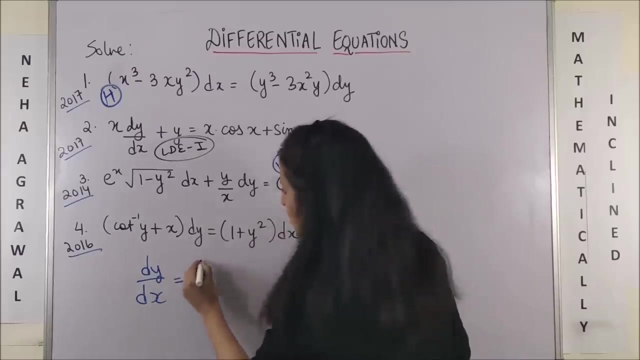 and there is already a detailed video on the same. Please make a note. Ok, so this was variable separable. Now let's move to the fourth one. So here your dy by dx is going to be, as I can see, 1 plus y square. 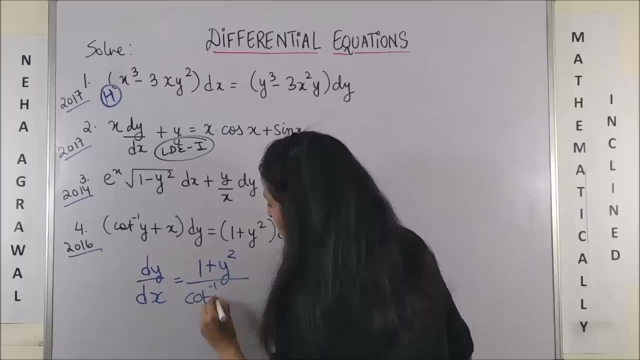 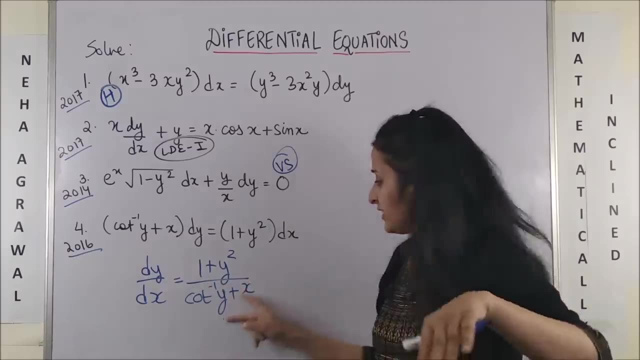 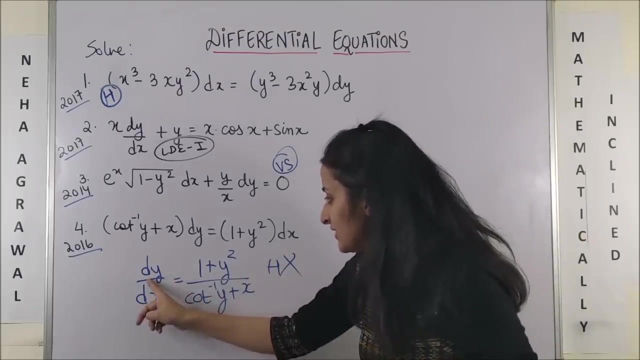 upon cot: inverse of y plus x. Ok, Again, constant term: degree 2, degree 1, degree 1.. So not homogeneous for sure. Now let's see variable separable. If I take this on this side, and even this one, I cannot get rid of x, See. 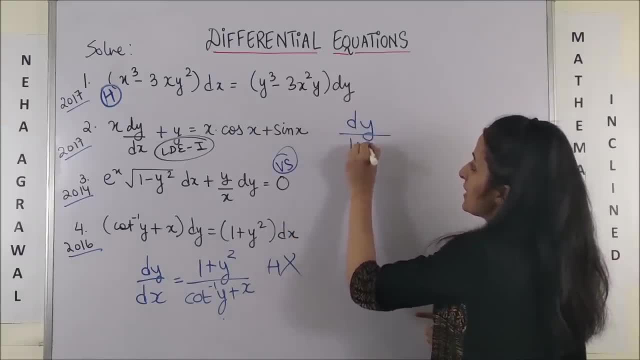 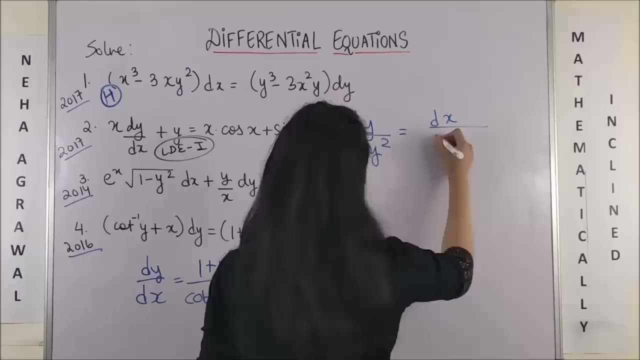 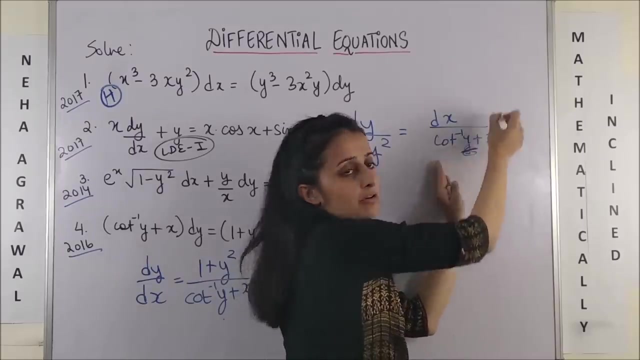 if I write this as dy upon 1 plus y, square Right On my right, I will have dx upon cot, inverse y plus x. Now this is sorted, but here I have the term containing y also. So definitely not your variable separable Linear. 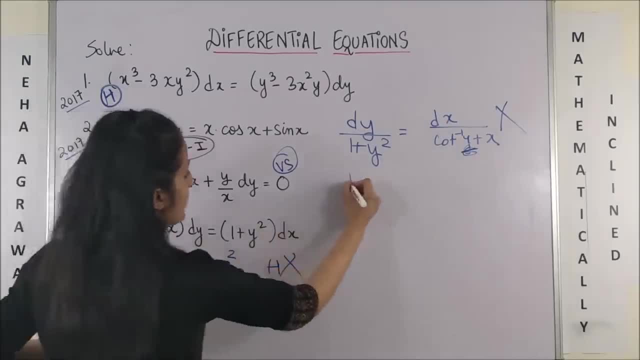 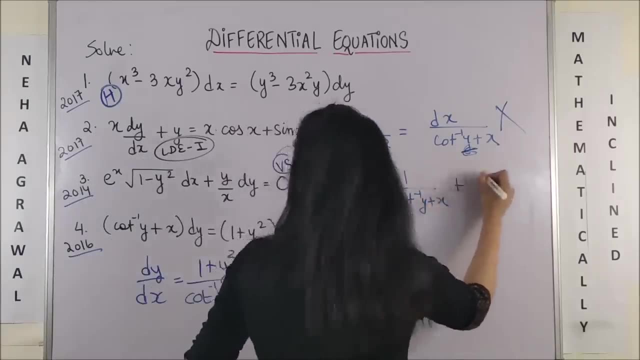 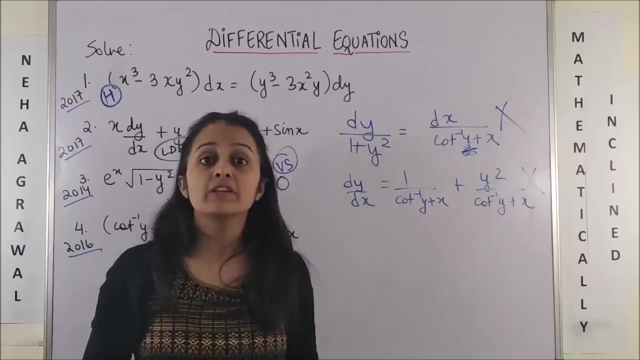 if I try to separate these terms, ok, I will get. dy by dx is equal to 1 upon cot inverse y plus x plus y, square upon cot inverse of y plus x. No, this doesn't even go with linear differential 1.. That means we have to now move to. 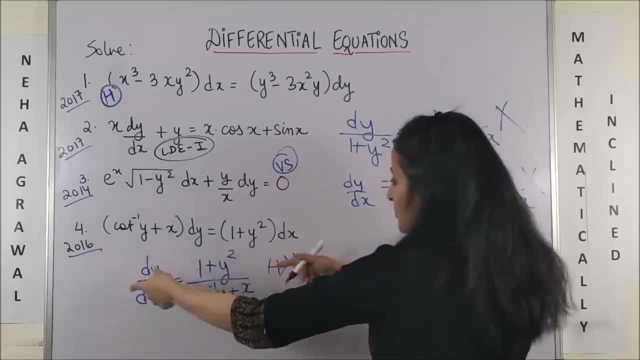 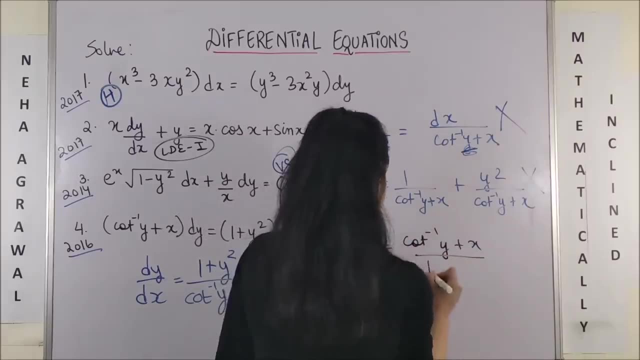 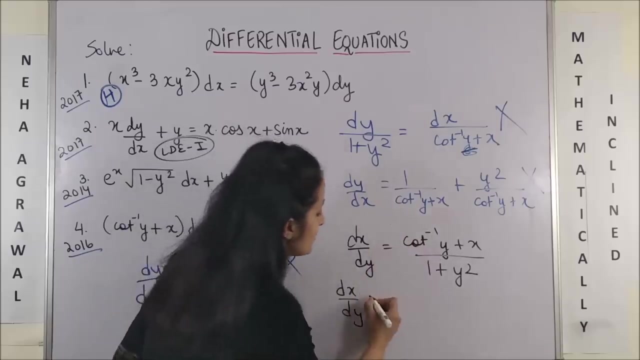 linear differential 2.. This means if I flip both the sides, so dx by dy is cot inverse of y plus x upon 1 plus y square, So this will be dx upon dy. If I separate them out, this will be plus and I will have minus 1.